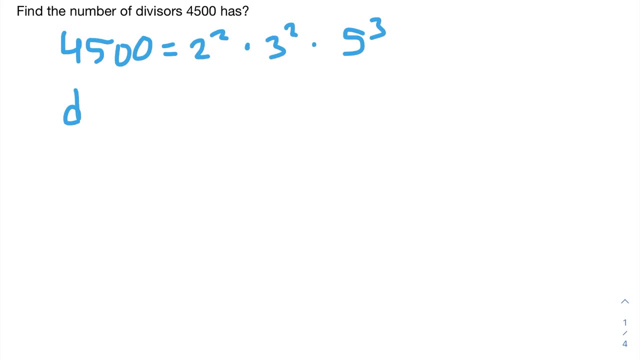 just call it: D of 4500 will divide 4500 evenly. So in other words, 4500 will be divisible by D if D is a divisor of 4500.. Now let's take a look at what D could be If D is equal. 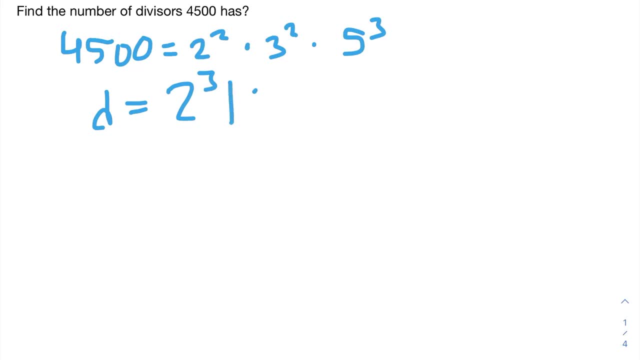 to 2 to the power of 3 times an integer k, then it can't be a divisor of 4500, because if D is a divisor of 4500, 4500 has to be divisible by D, And if we have 2 to the power of 3 in D, then we can never completely simplify this fraction. 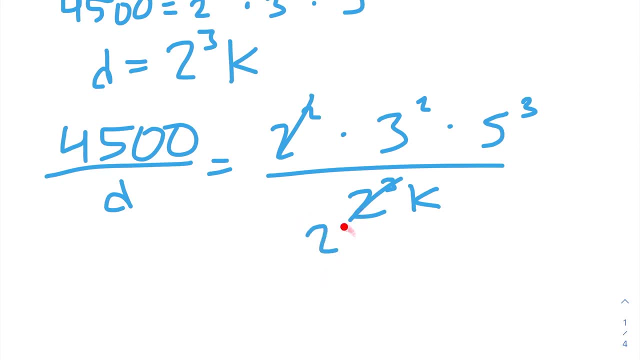 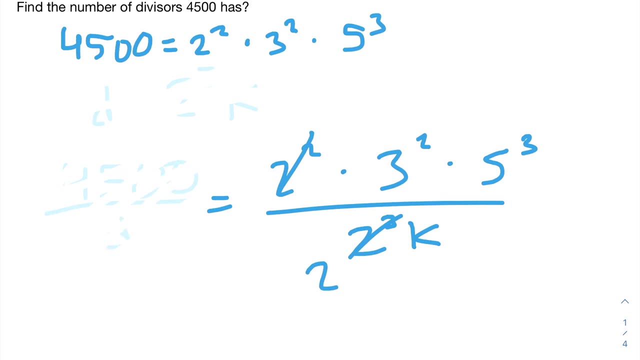 We will still have a 2 left in the denominator and we will have no way of getting rid of it. So if D is a divisor of 4500, it cannot have more divisors than 4500.. So if D is a divisor of 4500, it cannot have more divisors. 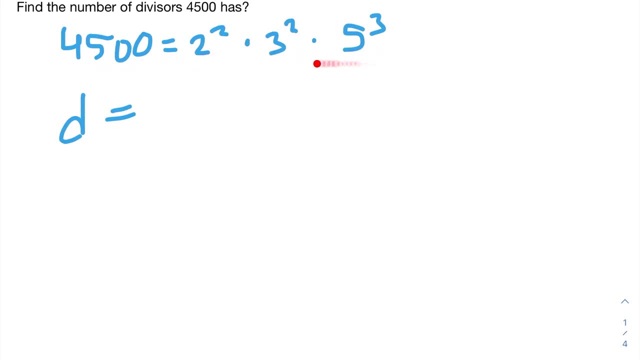 more factors of any of the primes in the prime factorization of 4,500 than 4,500 has. So d cannot have more factors of 2 than 4,500 has. That goes for any other prime that is in the prime factorization. 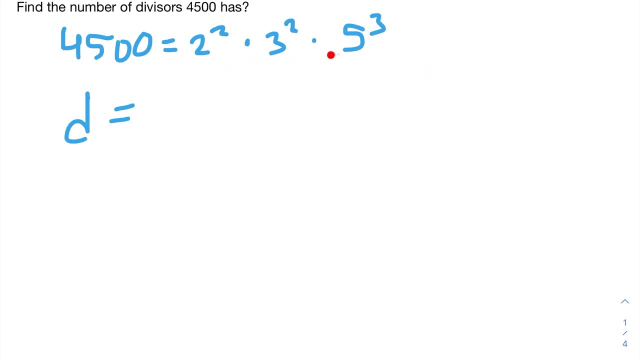 of 4,500.. So the same goes for 3 and 5.. Now, what if d is equal to 7n, where n is another integer? Well, in this case d also cannot be a divisor of 4,500. 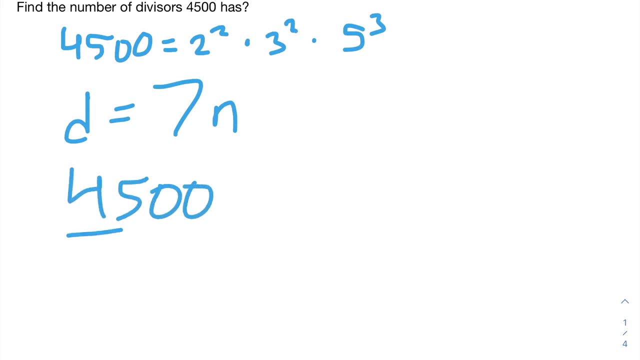 because there's no way to get rid of that 7. that will be in the denominator, And we can no longer simplify that because there's nothing to cancel out the 7.. So what did we learn from all this? Well, we learned that d has to be in the form of. 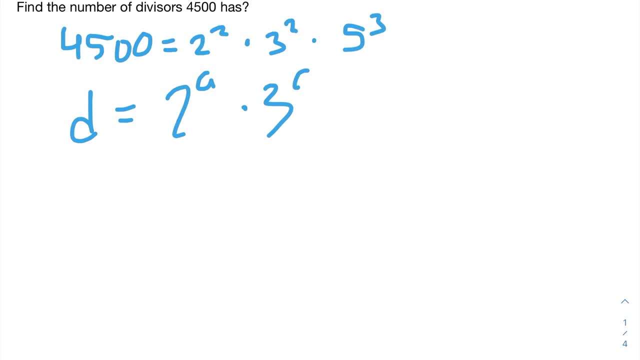 2a times 3b times 5c, where a is equal to 0,, 1, or 2,, b is equal to 0, 1, or 2, and c is equal to 0,, 1,, 2, or 3.. 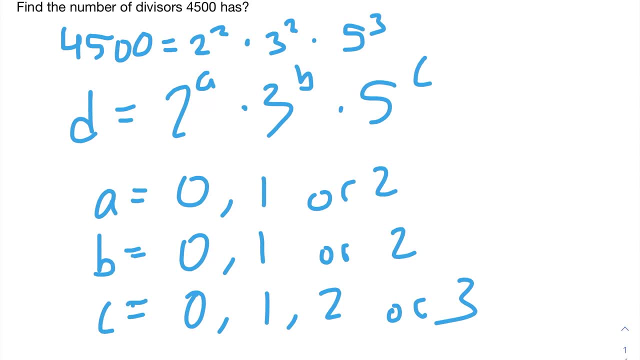 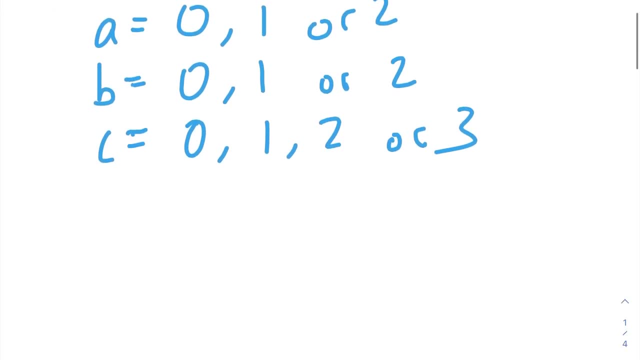 So now we're going to use a little bit of combinatorics to find out how many divisors 4,500 has. Any divisor d can either have 0, 1, or 2, 2s, so it can have 3 different numbers of 2s. 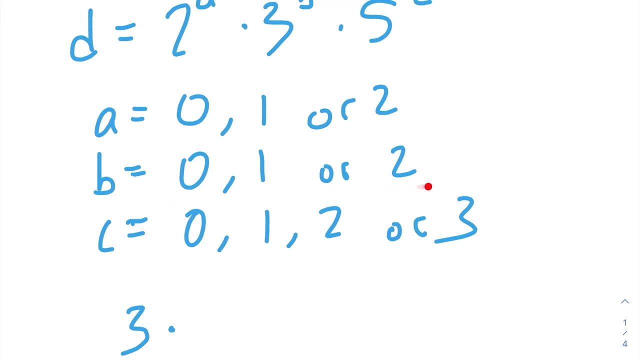 Each different value of d could have 0,, 1, or 2, 3s. So we have 3 different options for how many 3s we want, And each different d can have 0,, 1,, 2, or 3,. 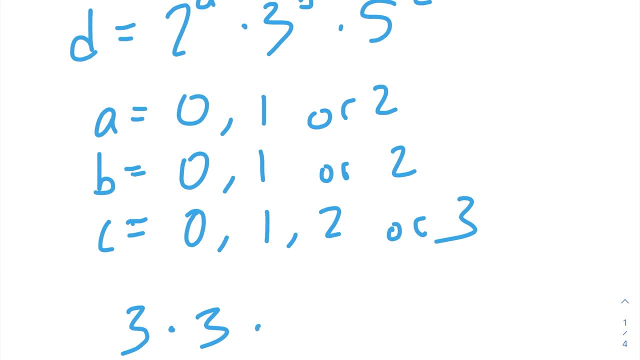 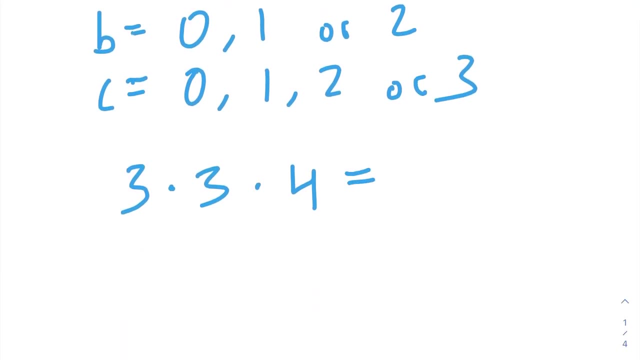 number, uh, 3, 5s. So we have 4 options for the number of 5s in each divisor of 4,500.. If we multiply all this together we'll get 36.. So 4,500 has 36 divisors. 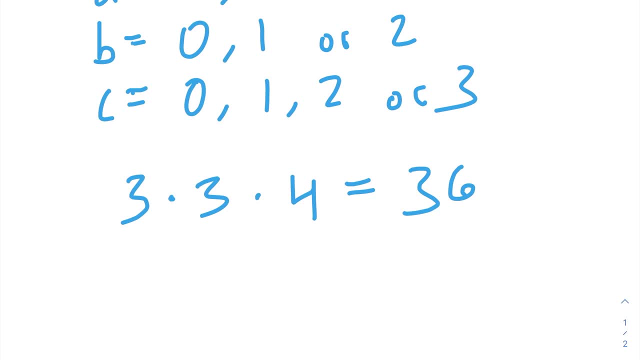 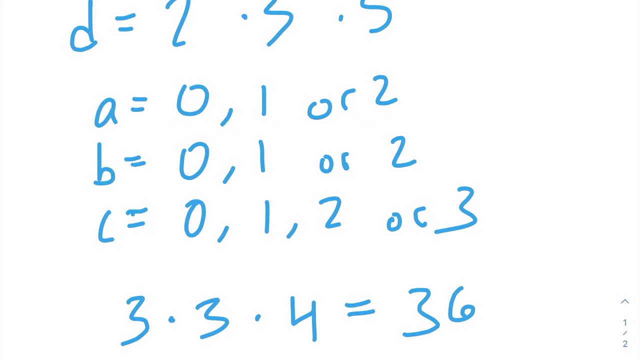 Now let's try to generalize this a bit more. We said that a can be equal to 0,, 1, or 2.. So, in other words, it can be equal to any integer between 0 and 2.. b is equal to 0,, 1, or 2,, which is also. 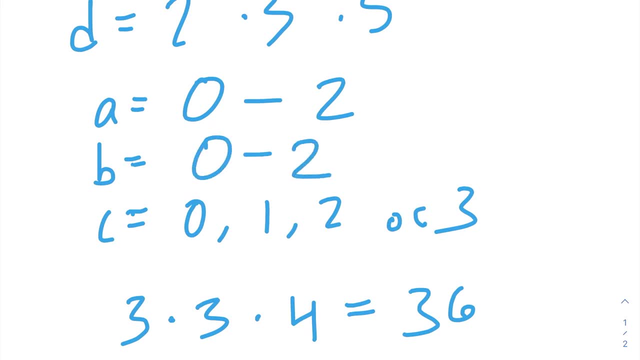 any integer between 0 and 2.. c equals 0,, 1,, 2, or 3, which again can be expressed as any integer between 0 and 3.. Now all we have to do is count how many integers there are. 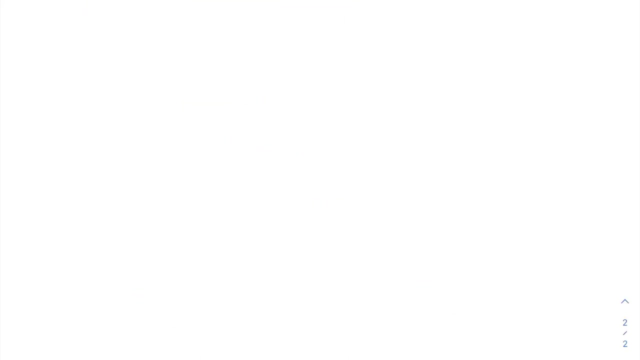 between 0 and 2.. We know there are n plus 1 integers from 0 to n, So there must be 2 plus 1 integers from 0 to 2,. 2 plus 1 integers from 0 to 2,.